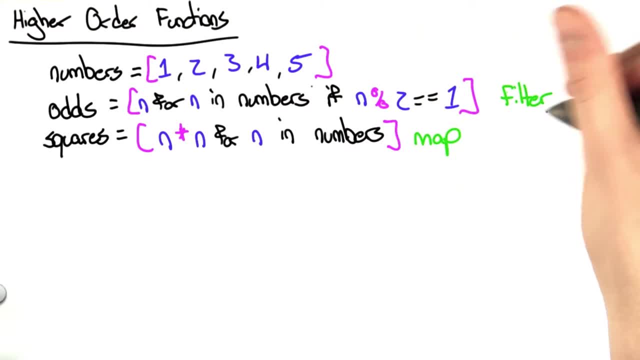 This is usually referred to as a filter and this is a map. When we're filtering, we take in a list of numbers and some criteria and only return the numbers that satisfy that criteria. In a mapping we take a list of elements and some operation. 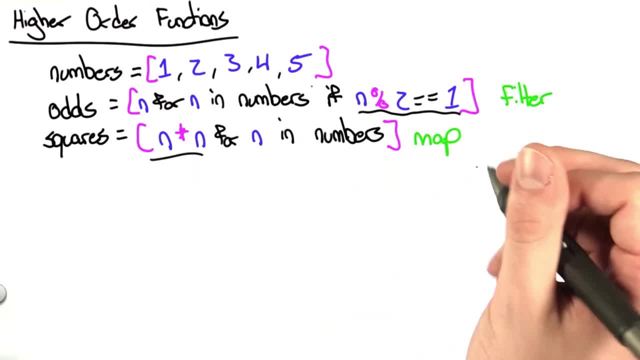 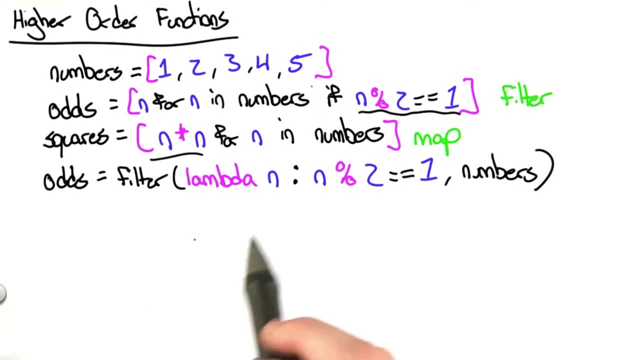 and we perform that operation on each element. Python actually gives us built-in functions to do this. Another way to write odds is to use the built-in function, where we give in two arguments. The first is a function that we create anonymously using the lambda notation. 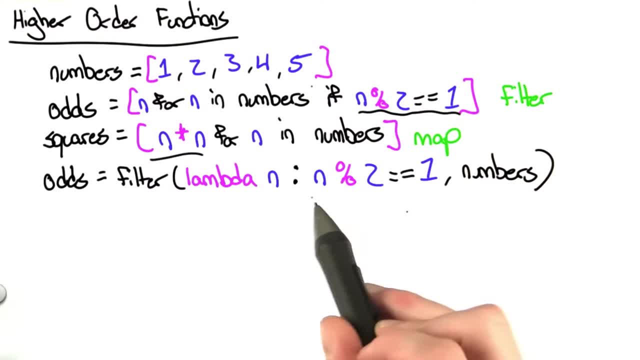 that returns true or false: true if n is odd and false if n is even. The second parameter is the numbers Filter is going to return all the numbers that, when inputted into our first parameter, this function return true. Here's how we generate the squares using the map operation. 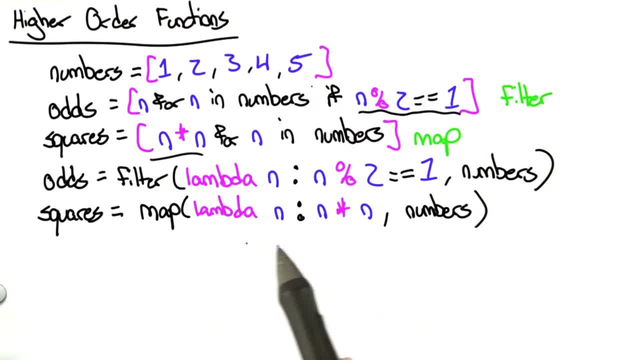 We pass in two parameters, just like we did with filter, where the first one is a function, the second one is a list, and map returns a new list. that is the result of applying each element in numbers to the first parameter that we gave the function. 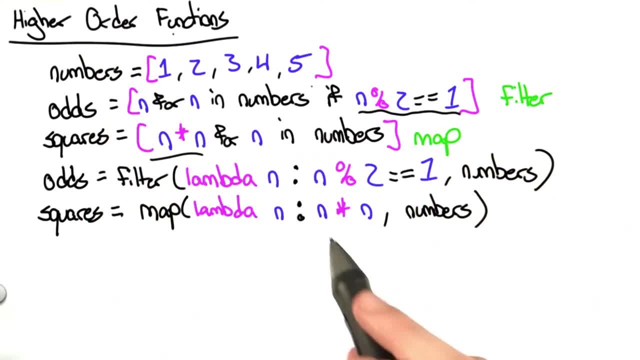 This problem asks us to create what is known as a higher order function. That is, we're going to create a function that generates a function that saves us time from having to repeat this first part of the filter and the map every time we want to use the same operation. 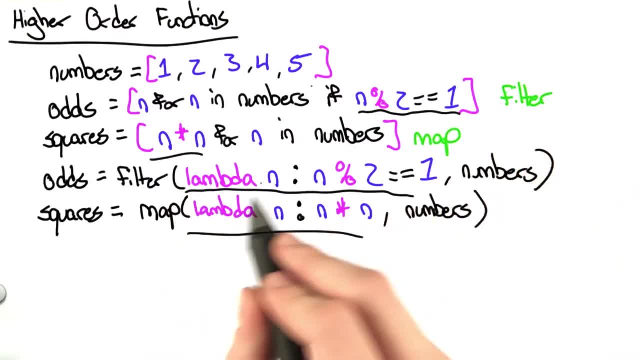 Ideally, instead of writing filter of lambda n n mod 2 equals, equals 1, we're just going to create an odd filter Here. our filter maker creates a new function that takes in one parameter numbers and applies filter in the same way as we have up here. 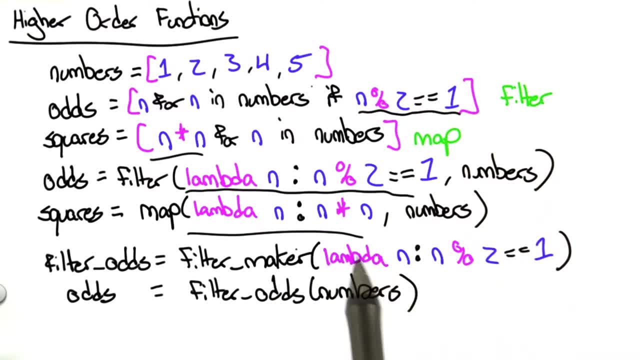 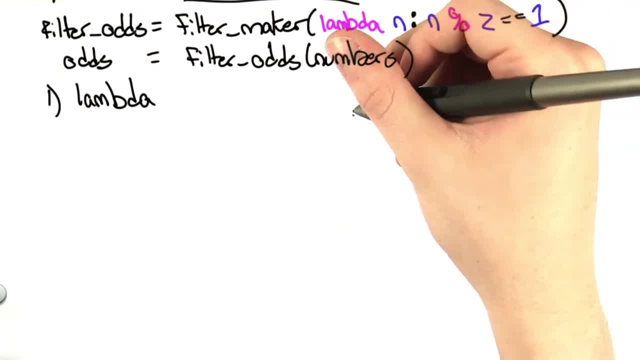 because we've already passed in to the filter maker the function that we want to use filter on. There are two ways you can solve this. The first would be using the lambda notation and the second is using inline function defines. Here we're creating a function using lambda. 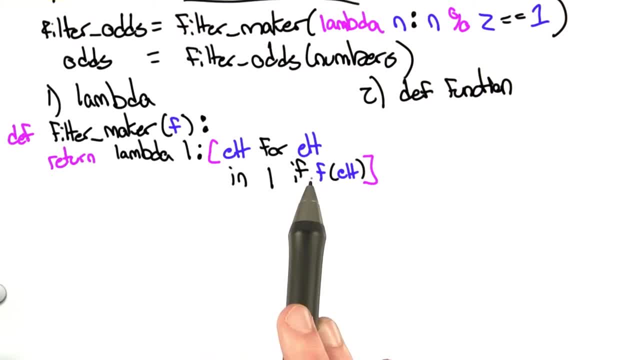 That's what lambda does. It's a function that creates a function. That is a list comprehension where, for every element in our list, which is the one parameter into our lambda function, l, we're going to leave it in the new function created by this list comprehension.